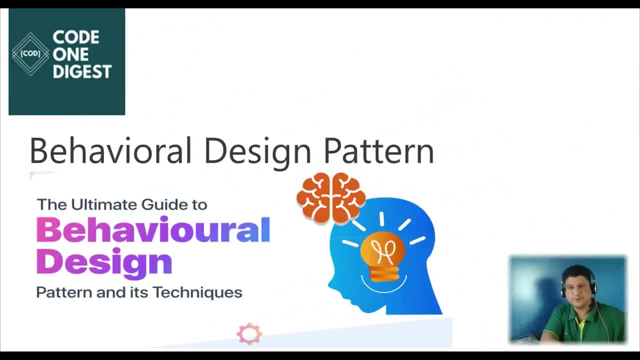 Hello, good morning friends. Welcome back to your favorite channel, Code One Digest Today. in this video I'll explain what is behavioral design pattern and where to use behavioral design pattern in our project. I'll also show the Java code implementation of behavioral design pattern. At the end we'll discuss the benefits of behavioral design. 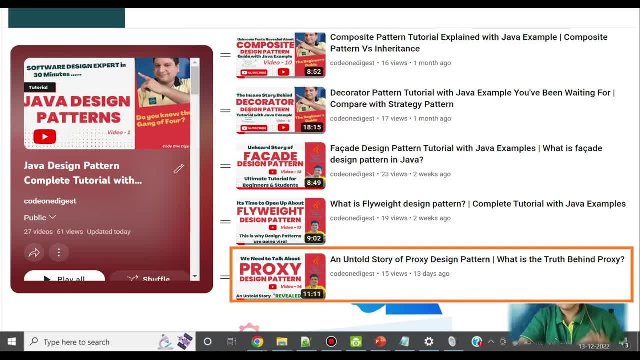 patterns. Friends, in the previous video we discussed about proxy design pattern. Can you explain what is proxy design pattern and where to use it? Please reply your answer in the comment section. If you have not seen the previous video, so I recommend you to. 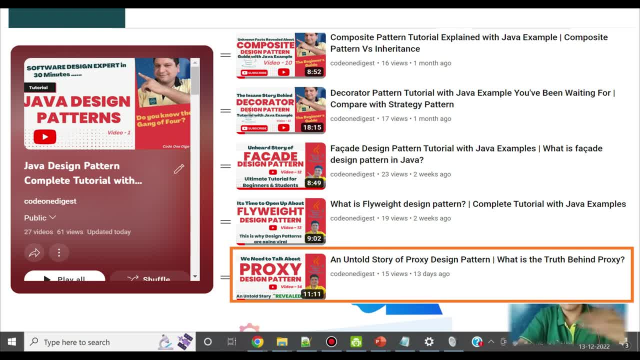 go and see the video. The video link is given on your screen and also provided in the description section. Just to recall the proxy design pattern. proxy design pattern provides a simple object to access the complex object. This is to avoid the need of creating an expensive object. So for more information, please see the. 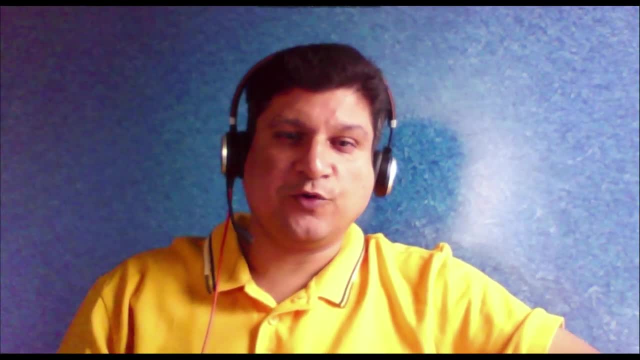 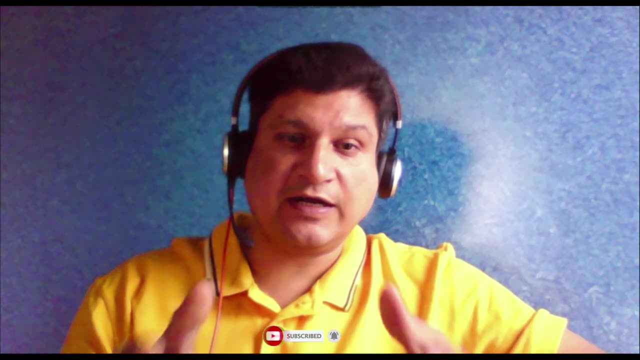 previous video: Friends, before we proceed in this video, I want you to subscribe my channel to grow. Code One Digest: family Friends. I'm creating a lot of quality contents for you, but I'm not getting subscribers. I want you to like, share and subscribe my channel. 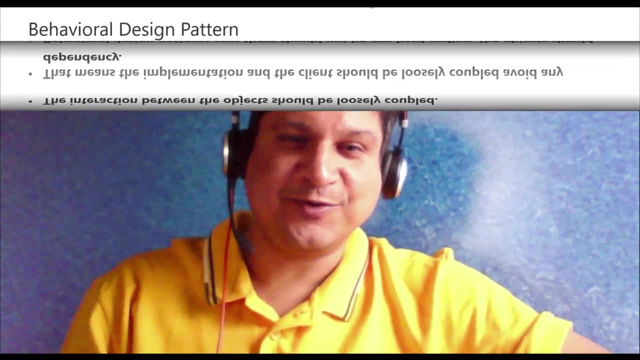 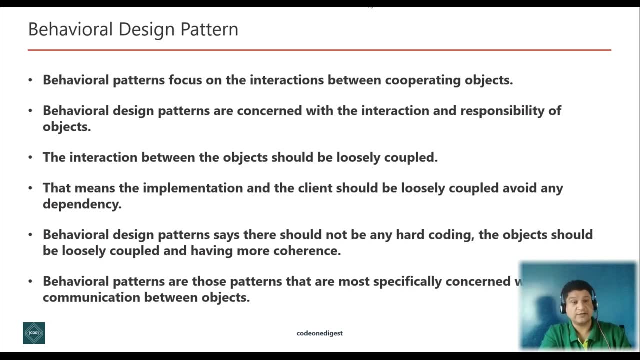 so that I can grow Code One Digest family. Thank you. Okay, let's start with the behavioral design pattern. Behavioral design pattern focuses on the interaction between the cooperating objects. Behavioral design patterns are concerned with the interaction and responsibility of objects. Behavioral patterns: 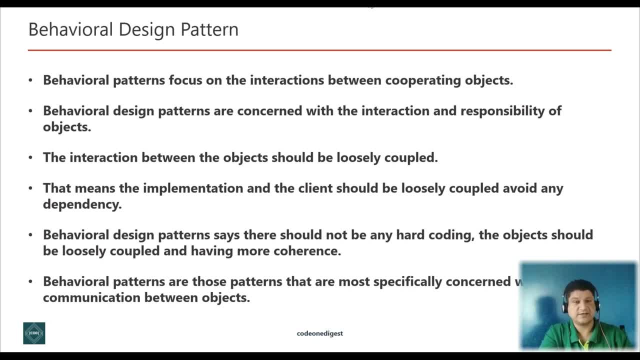 only concern about the communication between the objects. The interaction between the object should be in such a way that they can talk to each other easily and should be loosely coupled. That means the implementation and the client should be loosely coupled to avoid any hard coding or dependencies. The interaction between the cooperating objects are loosely. 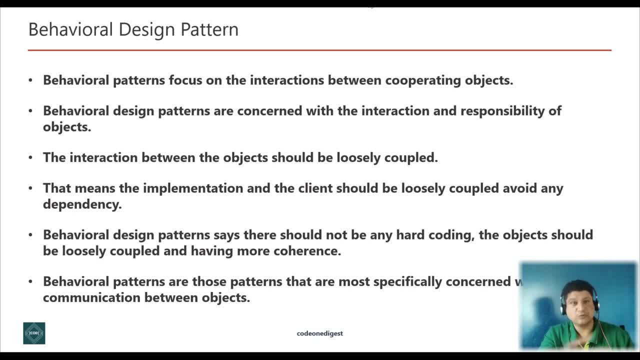 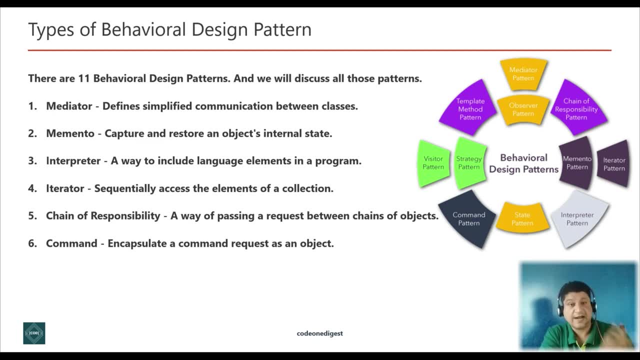 coupled and the loose coupling is the key to the entire architecture. Friends, there are 11 different types of behavioral design pattern and we will discuss all these patterns in coming videos. Now let's give a quick glance to all these design patterns. First is mediator design. 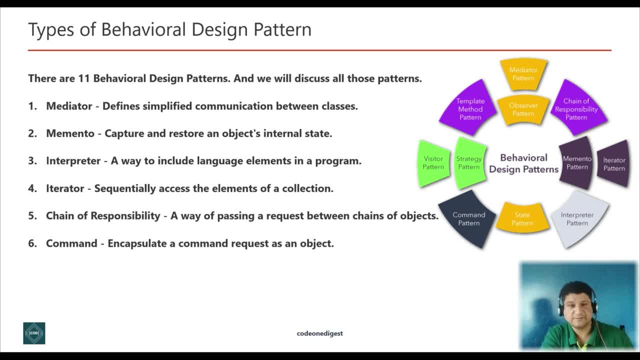 pattern that simplifies the communication between the classes of objects. As you can see, all the design patterns are commensurate. It is particularly important to see how the 2. Memento, 3. Interpreter, 4. Iterator, 5. Chain of Responsibility. 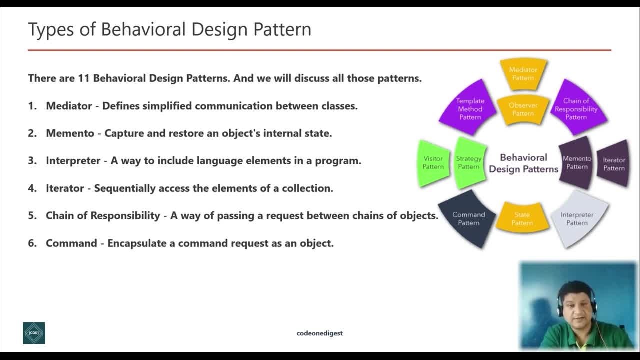 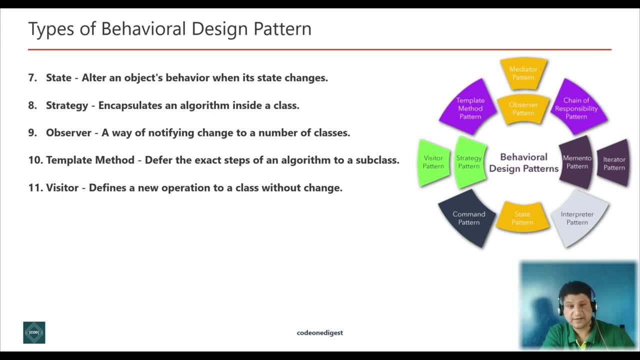 6. Command Design Pattern, 7. State Design Pattern, 8. Strategy Design Pattern, 9. Observer Design Pattern, 10. Template Design Pattern. 11. Visitor Design Pattern. We will see all these patterns in details in coming video with java code implementation. 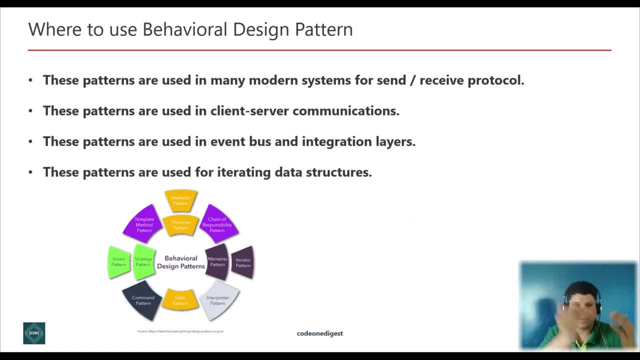 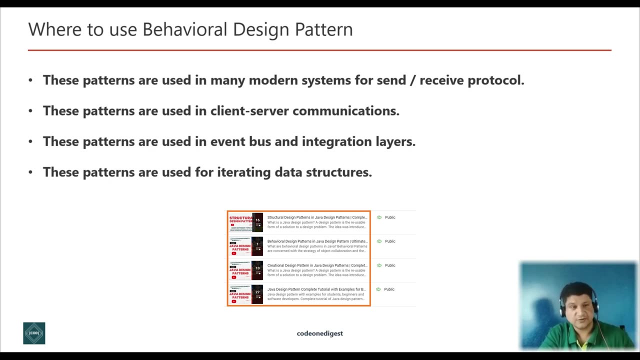 So, friends, the very first question strike to our mind: where to use behavioral design pattern? so these patterns are very useful in many modern systems, wherever we are sending or receiving messages. so there are multiple protocols which uses these behavioral design patterns for interaction, for communication. these patterns are used in client server communication. 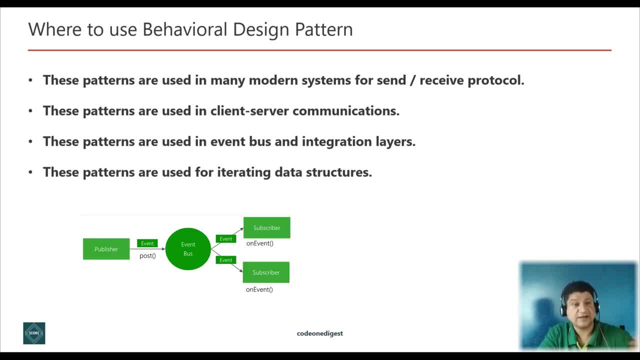 and also in event buses, in integration layers, middleware and so on. these patterns are used for iterating the data structure and so on. so this is very useful design patterns where the objects are involved and interacting with each other, how they are communicating with each other, transferring the information from one object to other object. 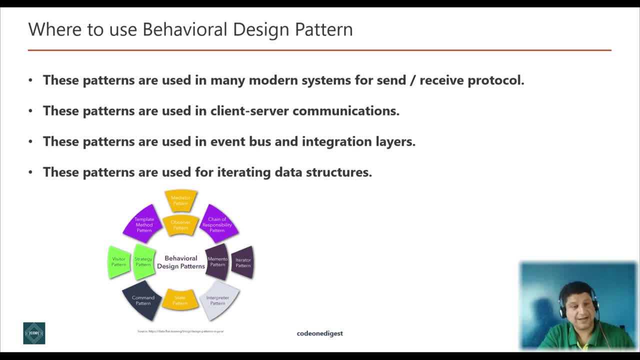 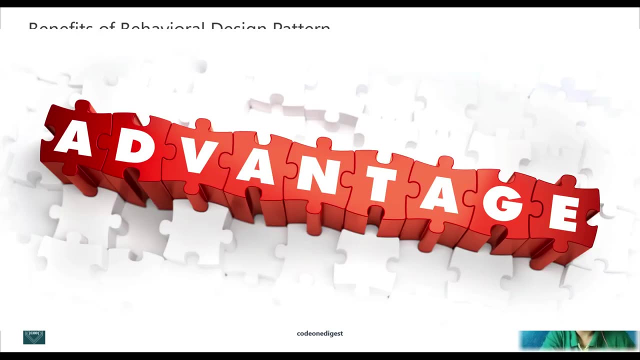 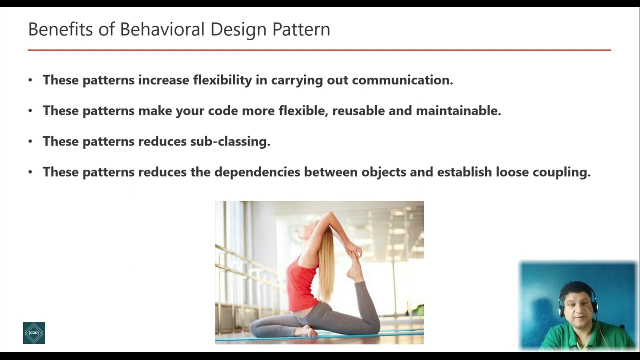 so there are various ways to do it and we will see all of those methods in coming videos when we discuss all these patterns in detail. so, friends, what are the advantages of behavioral design pattern that we get? so this pattern increases the flexibility in carrying out communication. this pattern makes your code more flexible. 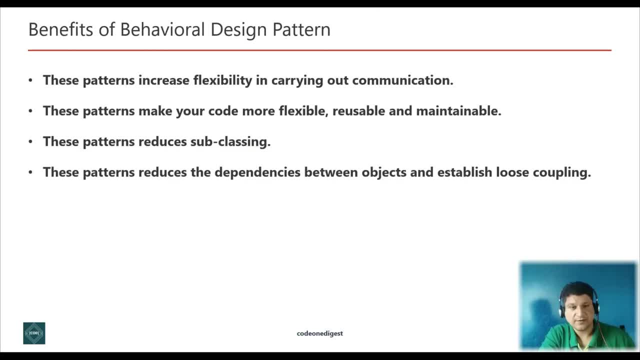 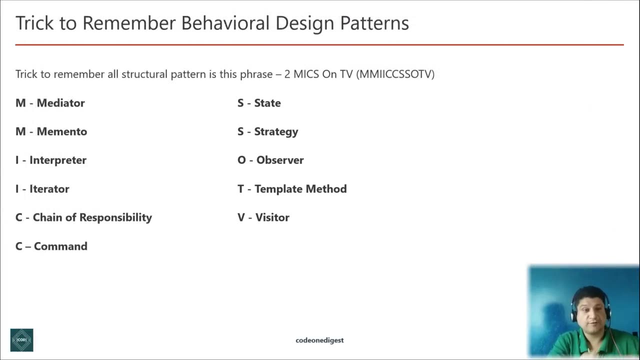 reusable and maintainable. this pattern reduces subclassing and this pattern reduces the dependencies between the objects and establish a loose coupling friends. you will wonder how to remember the name of all 11 behavioral design patterns. right, you don't worry, I'll teach you a trick to remember all these design patterns. 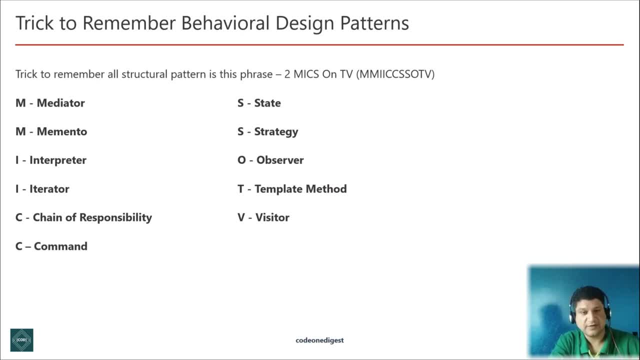 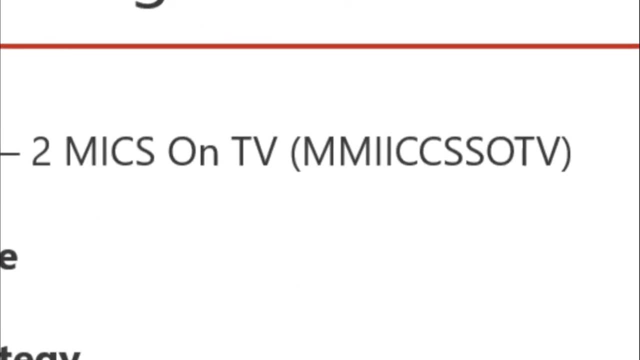 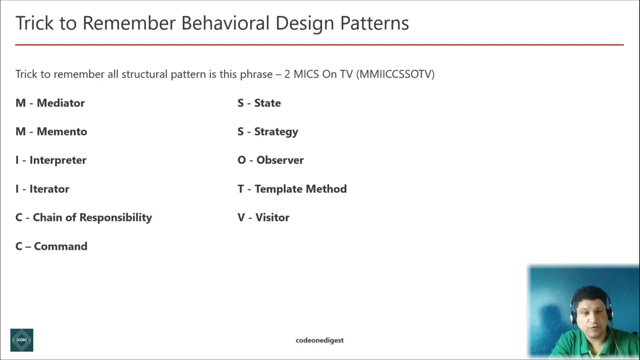 so the trick to remember all behavioral design pattern is this phrase: two mics on TV. if you remember this phrase, you will be able to recall all the behavioral design patterns. like two mics on TV. so M for mediator, then M for memento, I for interpreter. 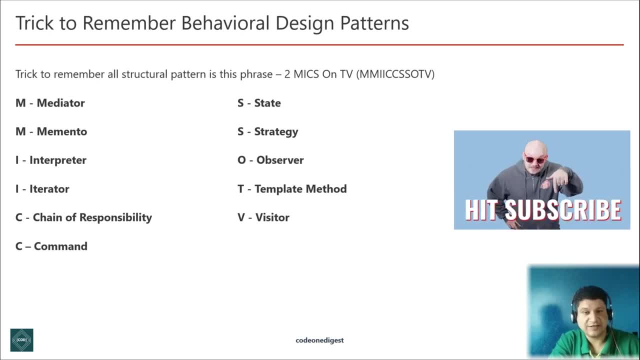 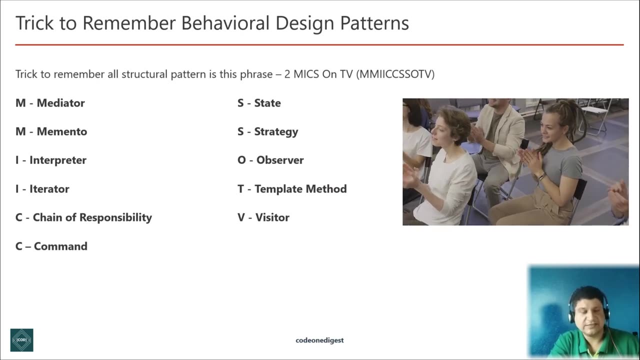 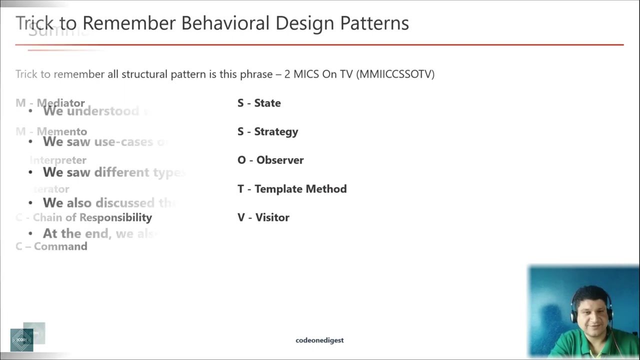 I for iterator, C for chain of responsibility, C for command, S for state, S for strategy, O for observer, T for template and V for visitor isn't easy to remember. just remember this phrase and you can recall all the behavioral design patterns right. ok, friends, now it's time for me to summarize. 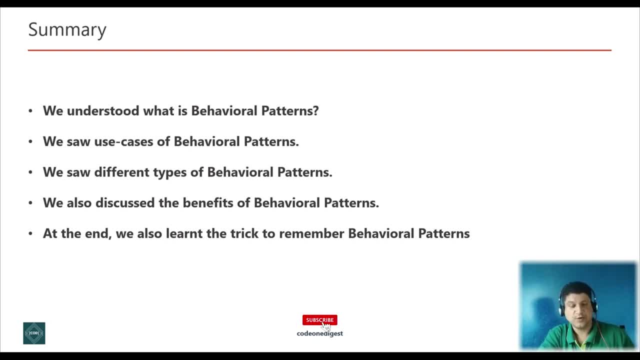 what we learned in this video. so we understood what is behavioral design patterns. we saw where to use behavioral design patterns. we saw the different types of behavioral design patterns- though we are going to discuss all those behavioral design patterns in detail in the coming video. we also discussed 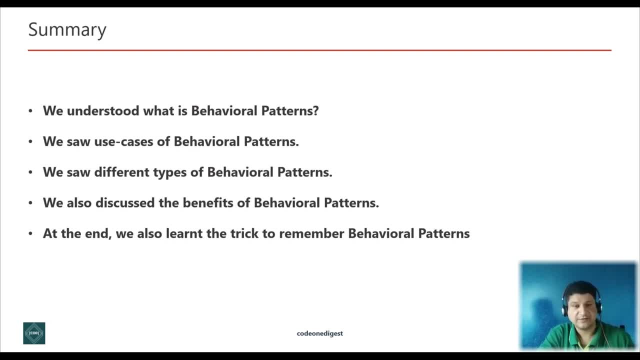 the benefits of behavioral design pattern and at the end, we also learned the trick to remember behavioral design pattern. friends, let me know if you are already using this behavioral design pattern in your project or you have seen a scenario where this pattern can be very useful. please reply. 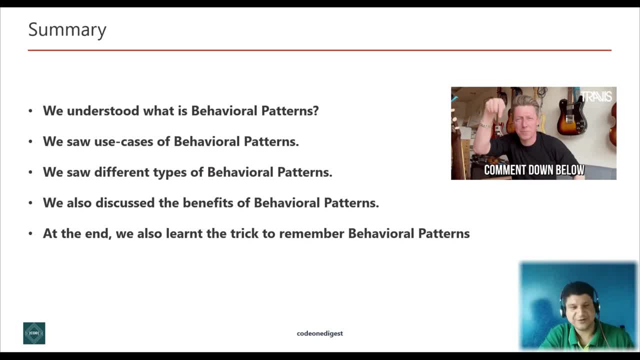 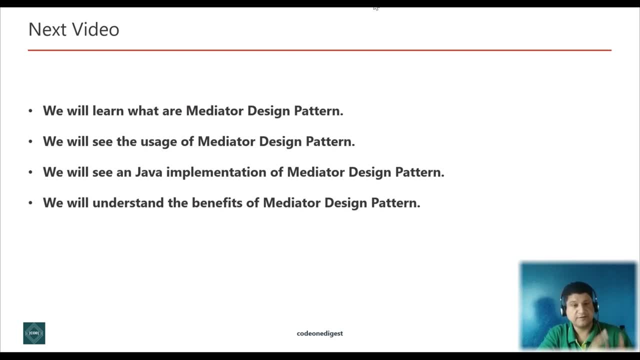 your answer in the comment section of this video. thank you, friends. in the next video we will cover our first behavioral design pattern, that is, mediator design pattern. we will learn what is mediator design pattern, we will see the usage of mediator design pattern and we will see a java implementation of mediator design pattern.